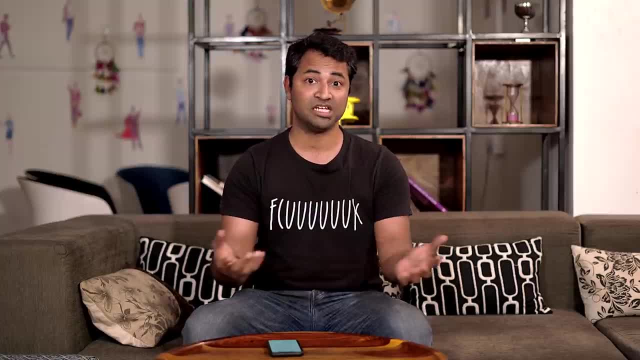 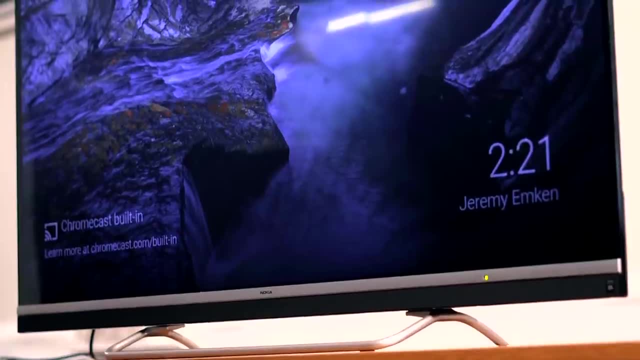 There are two things that most people look for while buying a television: hardware and software, of course. So in the hardware section you've got display and audio quality that most people generally look for when you're at Best Buy or Walmart or whatever, And there's 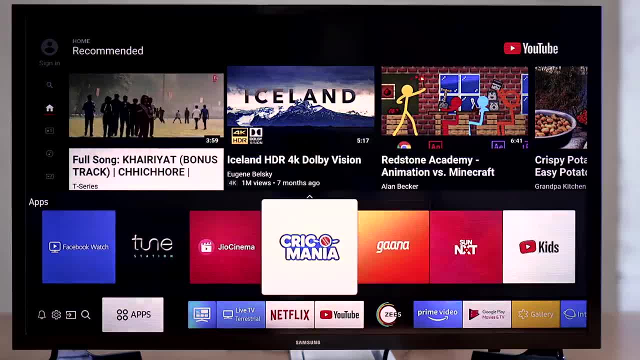 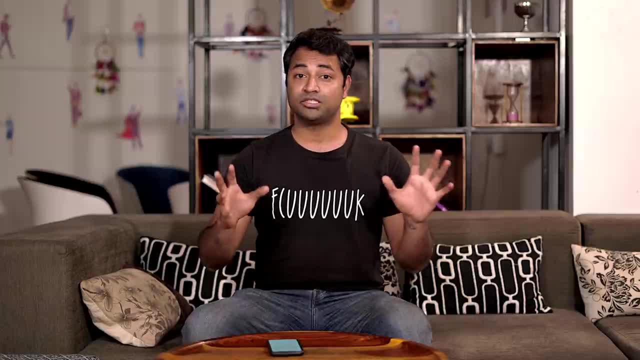 of course, software, which is lately becoming more and more important as you have to upgrade your software every now and then to keep up with most of the apps and all that jazz. So yeah, there's three major operating systems for most televisions. There's the webOS for 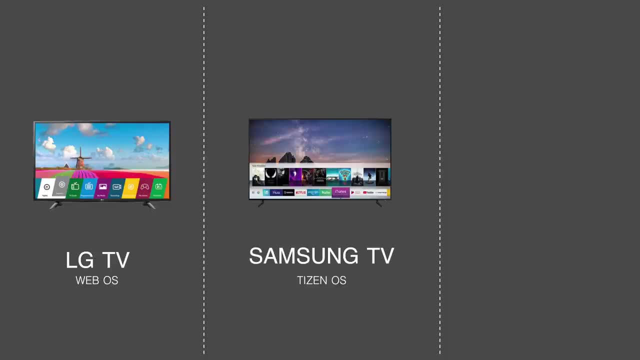 LG Smart TVs and the Tizen OS for Samsung Smart TVs and Android TV OS for most Android TVs out there. I mean, I know there's Fire TV OS and Roku OS for other operating systems, but that's for another day. So yeah, you're probably wondering which one's the best, or? 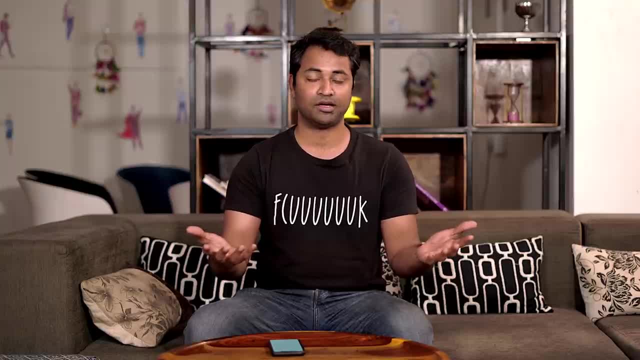 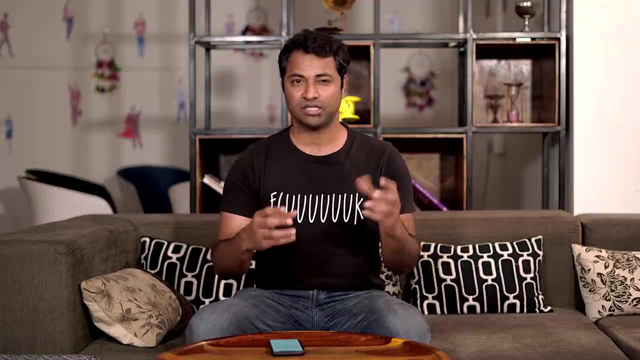 if you're considering buying a new one, you want to know about each and every OS out there. Most of the features in smart TVs are kind of similar. It's the only real difference that you actually see is in the little intricacies of the way the companies make those. 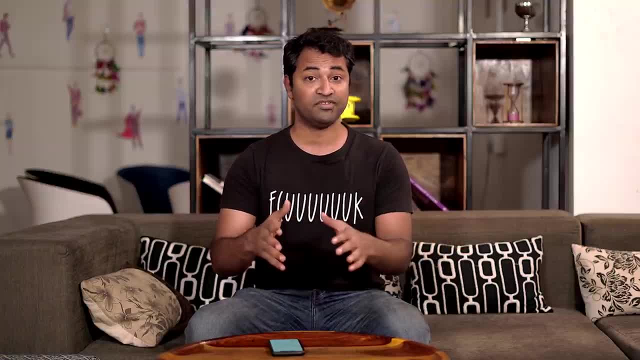 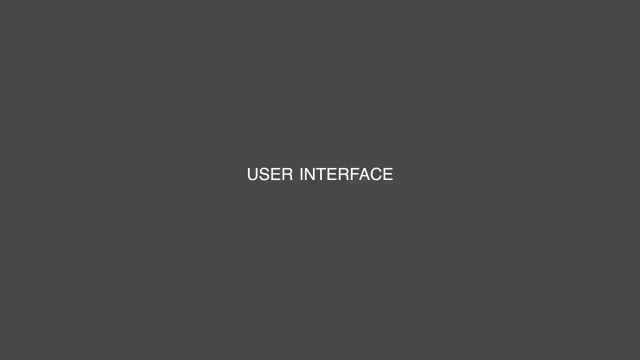 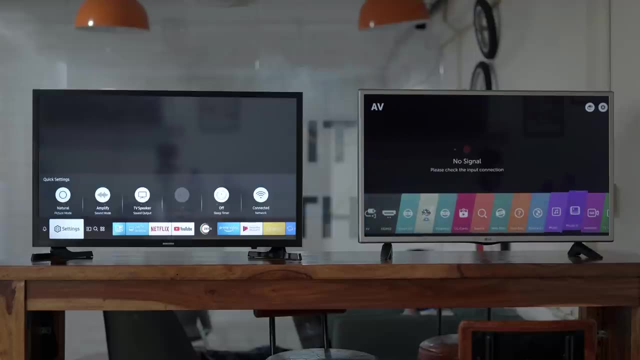 TVs. Let's see how you can actually differentiate one TV from another, starting with UI. In terms of interface, webOS and Tizen OS are quite similar. It's got a menu bar that you can gesture up from the bottom of the screen, which then contains a row of content. 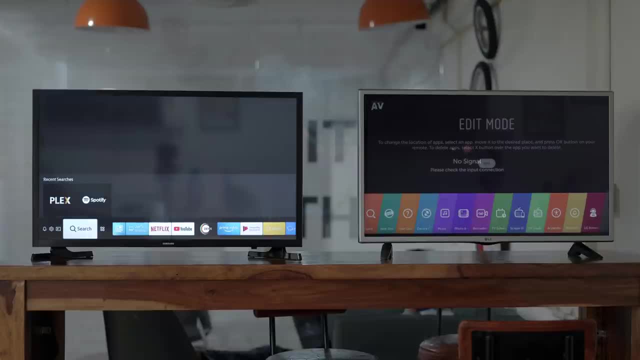 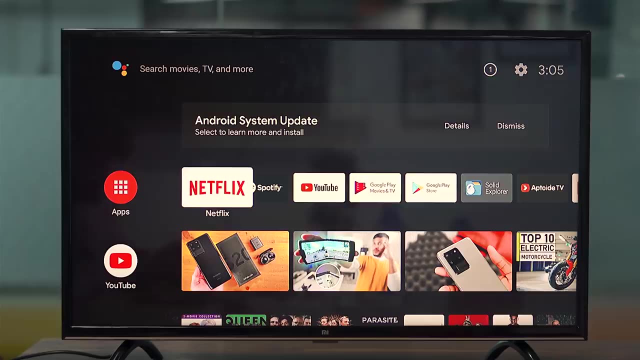 that you can scroll through And the icons are minimalistic. So, even if you are watching a movie or a TV show, you can still watch the content and navigate around. Android TV, on the other hand, takes the entire home screen with categories like voice. 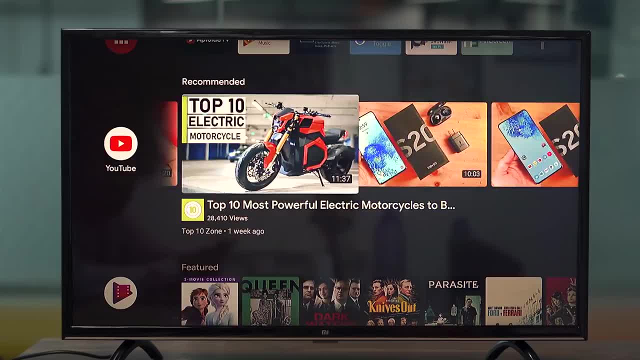 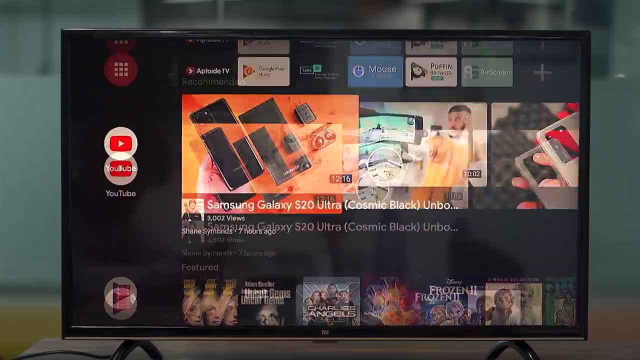 command search on the top, followed by popular apps and movies and TV shows that you're currently watching. You can't use the Android TV interface while watching your shows, Although, on the bright side, you can set a custom launcher on your Android TV, like the HAL Launcher. 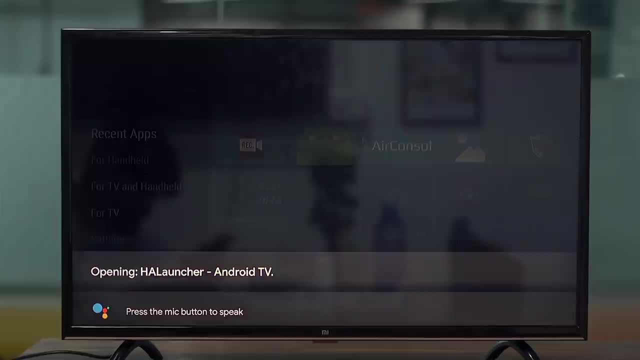 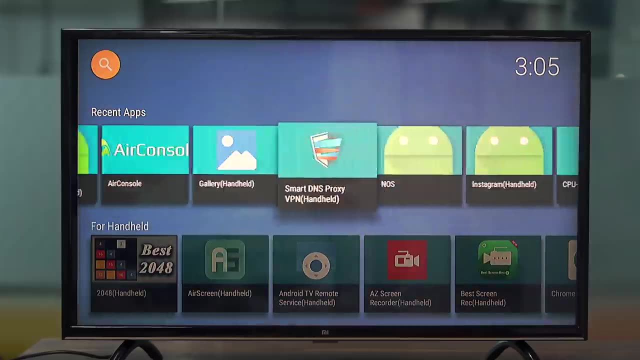 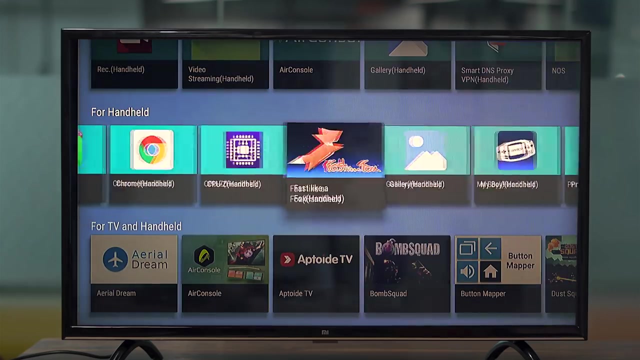 which lets you customize each and every setting. For instance, suppose I want to launch a handheld app like SmartDNS Proxy's VPN. To change my location in the regular launcher, I have to go install the sideloaded launcher to view it. But if you replace this with HAL, you move from this clutter of Hotstar and 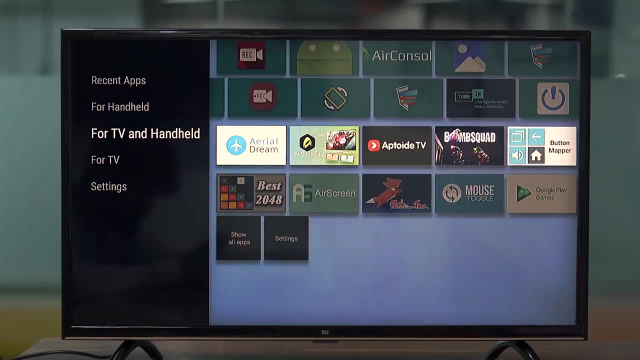 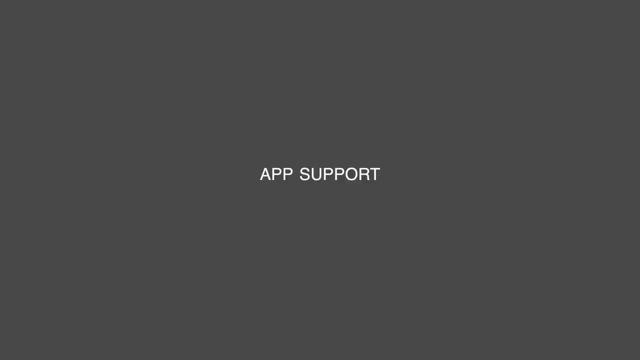 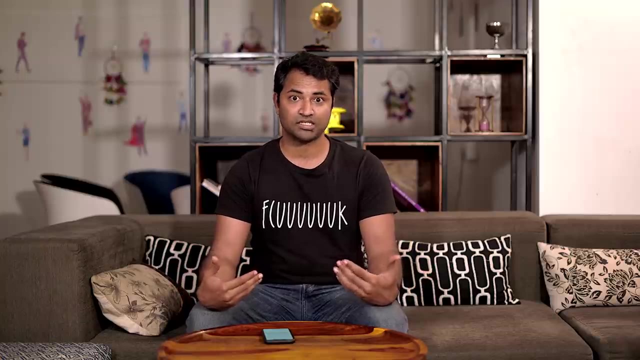 Netflix recommendations to a minimal layout that shows you all of your installed Android TV apps, as well as the handheld ones. Now, user interface is quite subjective, because I might like the minimalistic Tizen OS but you might like the Android TV. But you know what's not subjective: The number of apps, 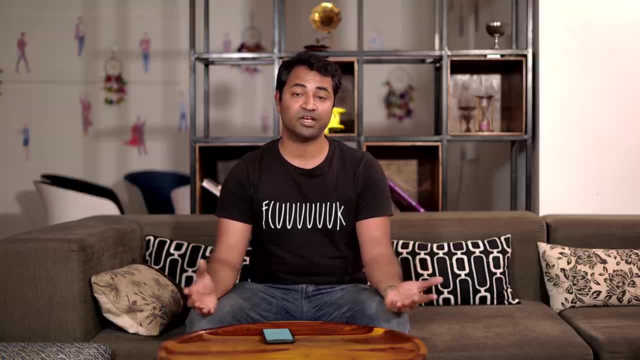 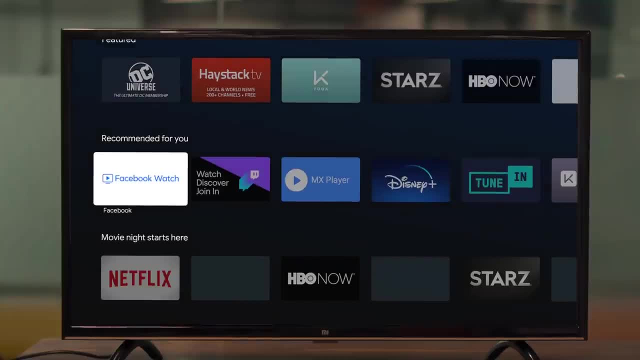 and app support. So let's take a look at the number of apps available for each and every operating system In app support. Android TV is the clear winner. You can easily install almost every application in the Play Store, And you can even sideload apps with the help of Aptoide TV, Like the. 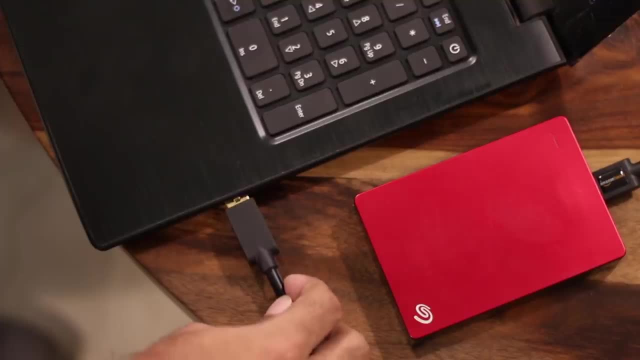 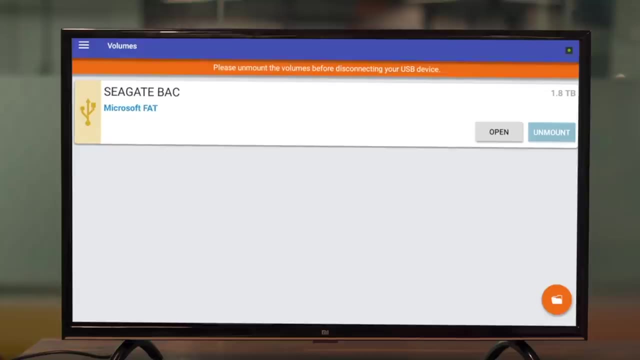 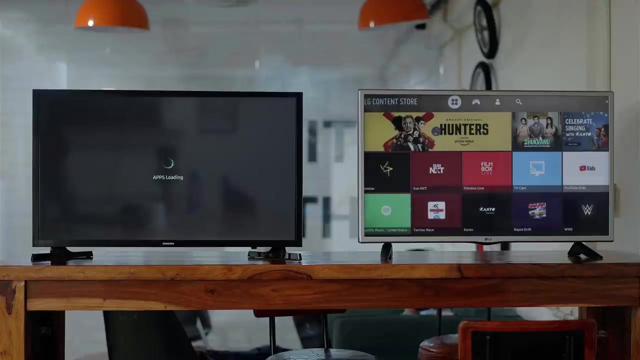 other day I wanted to read my hard disk drive, which was in exFAT format rather than FAT32, which is the one that most TVs read, So it uses the Microsoft exFAT NTFS Viewer to read all the content. On the other hand, Tizen OS and WebOS have basic apps like Netflix, Prime Videos, Disney. 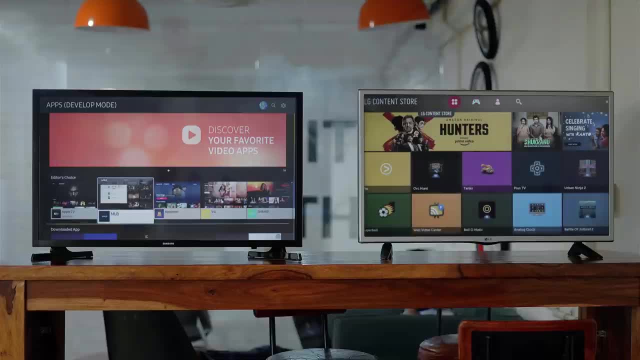 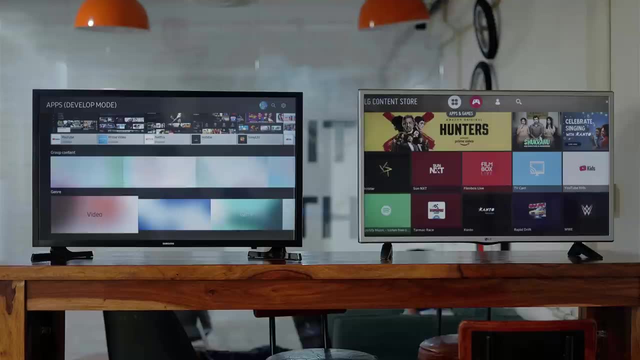 Plus and etc. It doesn't have apps like Notification Mirroring or exFAT View or you know useful stuff like that. And to make matters worse, you can't even sideload apps on Tizen or WebOS that easily, For example, if you want to use Hulu outside of the United States. 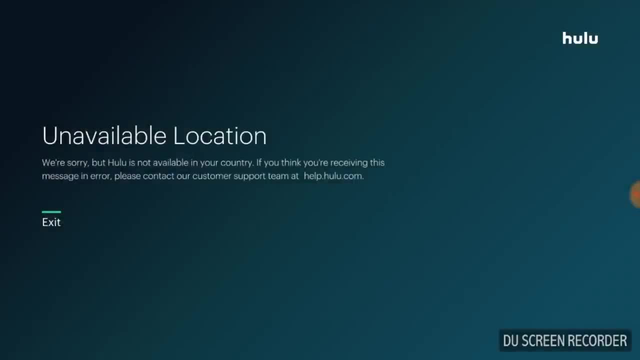 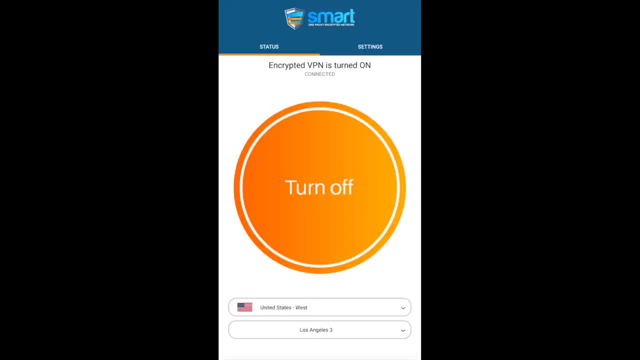 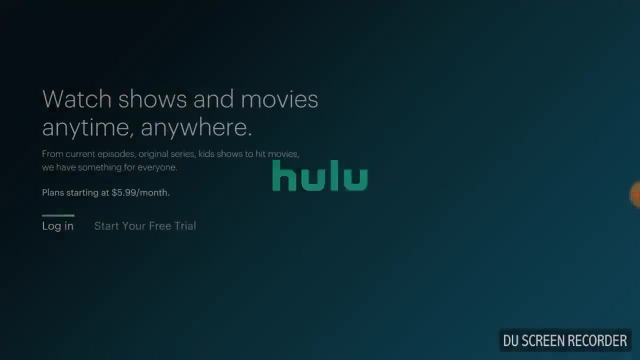 by default, you can't watch it in any of your TVs. However, on your Android TV, you can simply sideload the Hulu APK from the Aptoide TV store and then watch it on Smart DNS Proxy's VPN. However, if the Hulu app is not available in Tizen or WebOS, there's 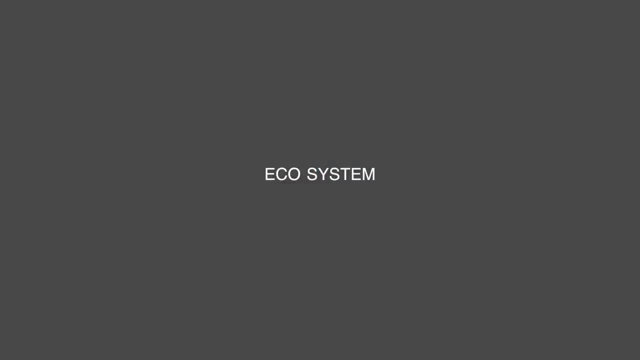 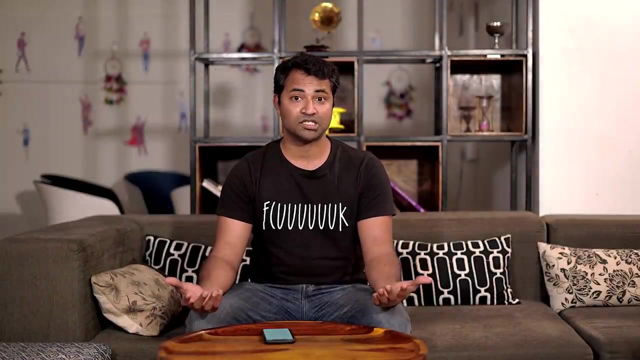 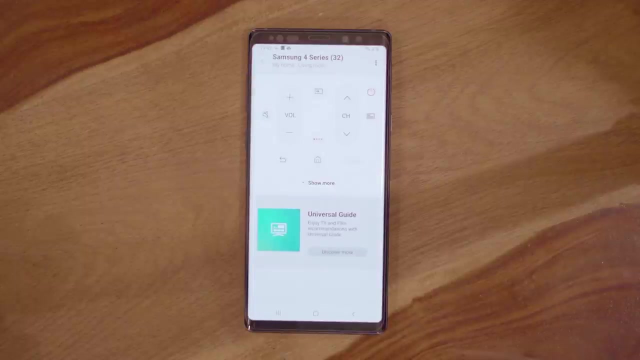 nothing you can do about it. Another important thing to look for while you're buying a Smart TV is the operating system. Tizen OS has an interesting feature. If you've got a Samsung Smart device like Note 9, you can not only control your TV with your smartphone app and type on your TV with your smartphone's. 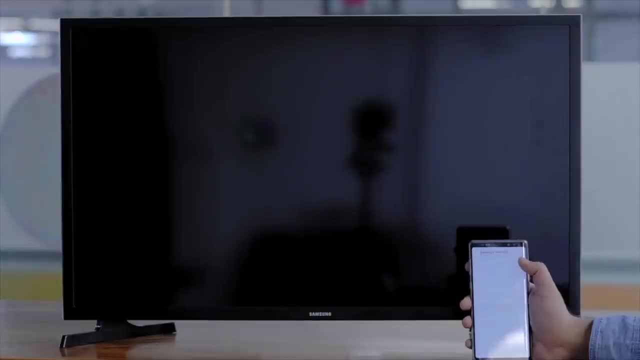 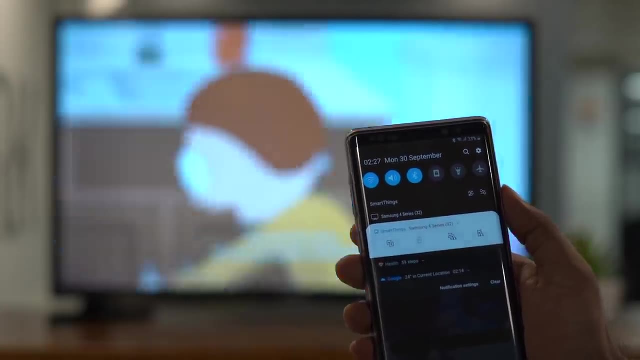 keyboard, but it even lets you turn on your Samsung Smart TV with your smartphone. That's something I've never seen in any other Smart TVs. One of my favourite features is private listening. Now you can listen to your television sound directly on your Samsung Smart phone. 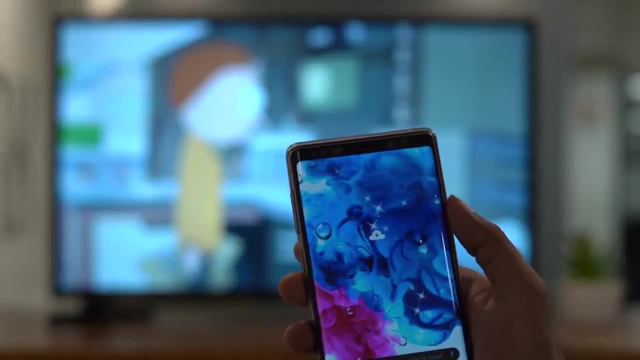 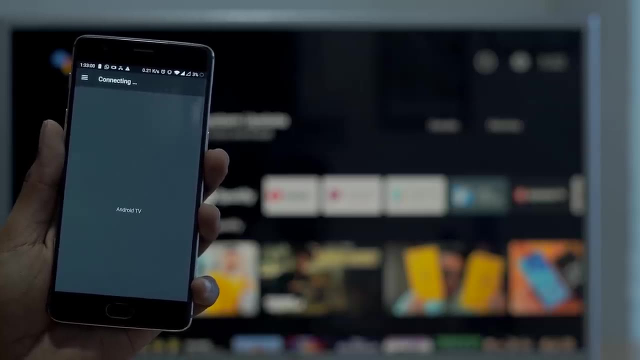 Check out the full video on Samsung TV tips and tricks if you're keen on knowing how to do all that aforementioned stuff. Moving on to Android TV, Many people know about Smart Remote to control your television and it works quite good if you have a touchpad, navigation controls or even Google Assistant. 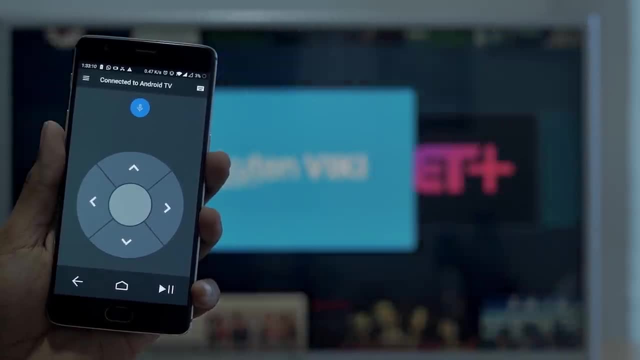 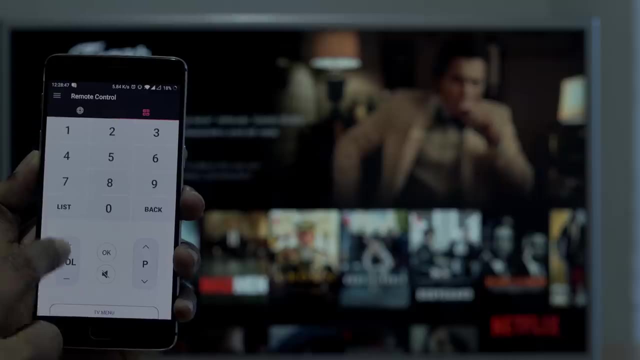 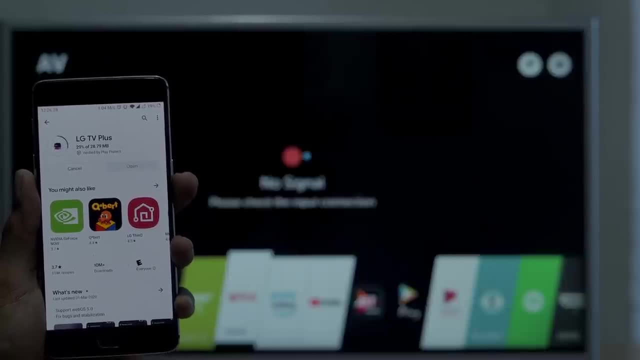 with the LG WebOS. You can also connect your smartphone with the LG WebOS. First of all, you need to download an app on your smartphone called LG TV Plus. When you open it, it will show your television, So choose your TV when that pops up, and then 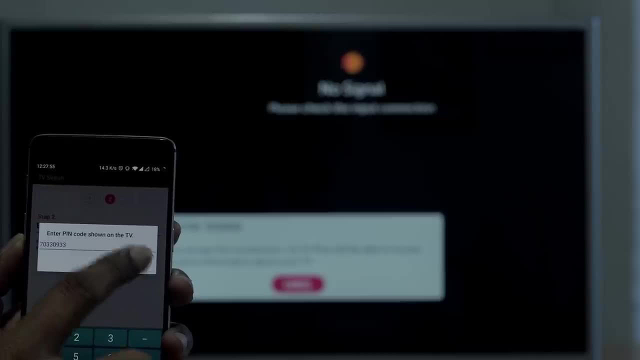 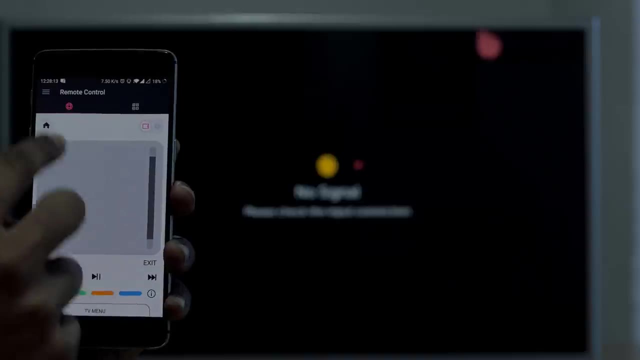 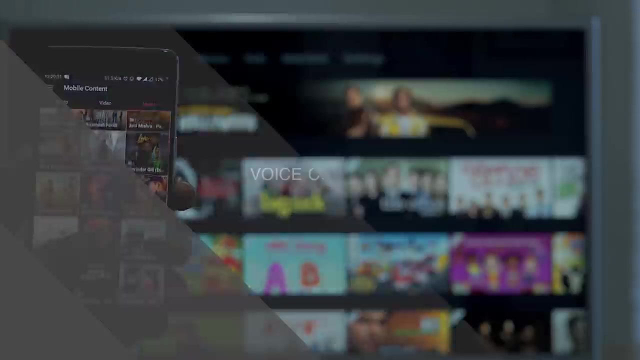 creates a time pin and enter that onto your phone. From my experience, this app works flawlessly. You can do everything that you do on your TV, like with a mousepad navigation, But the best part, though, is that you can directly play your mobile content on your TV without casting your device. 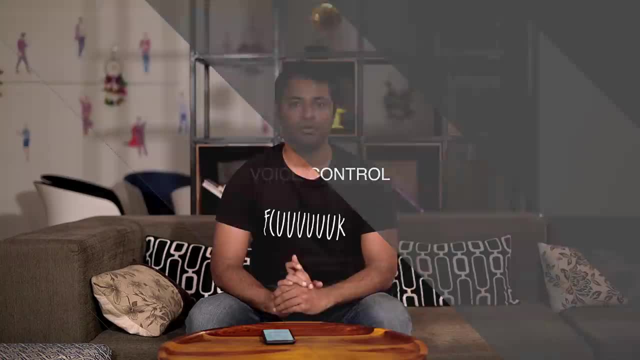 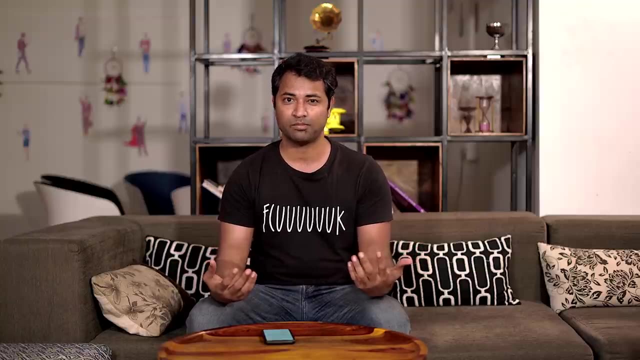 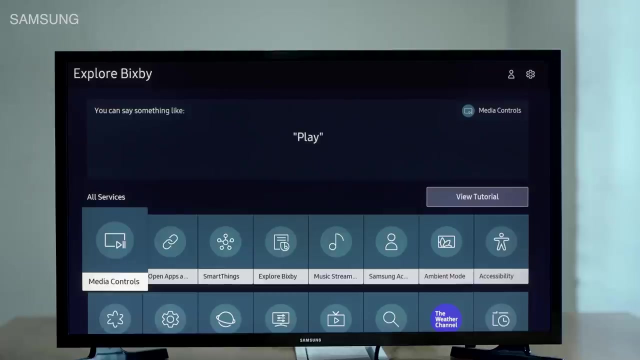 Pretty much all smart TVs now come with a voice control within it, like, say, Google Assistant or Bixby, but how good are they actually? For example, Tizen has a built-in Bixby engine that can recognize your words for changing TV settings and searching content. Tizen also supports the Google Assistant and Alexa for 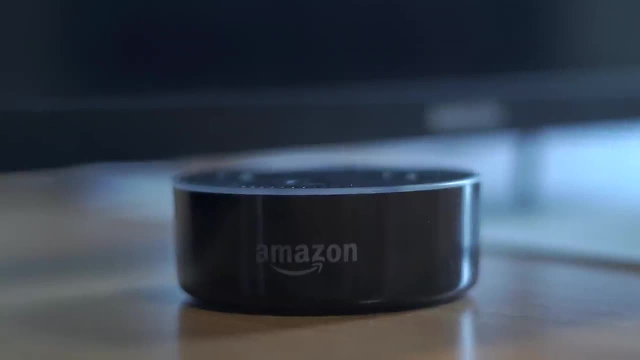 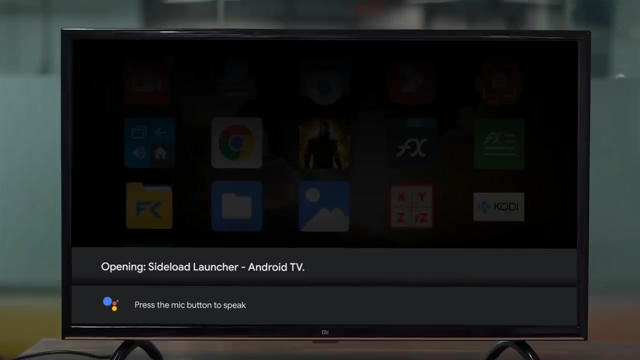 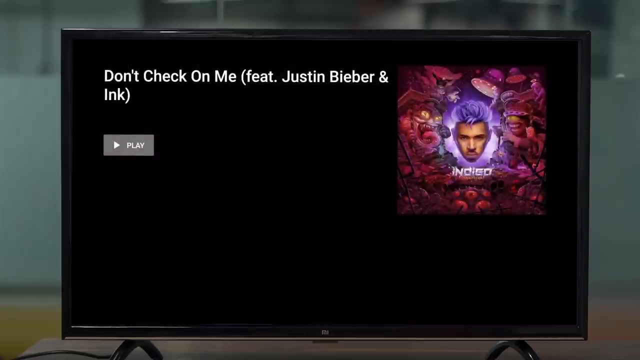 voice recognition, but only via external speakers. Android TV, on the other hand, lets you connect your phone to your smartphone with the LG Magic Remote. It lets you control your Android TV easily with Google Assistant. Most of your applications are just controlled via your voice that you can use to type with the help of Google Assistant. 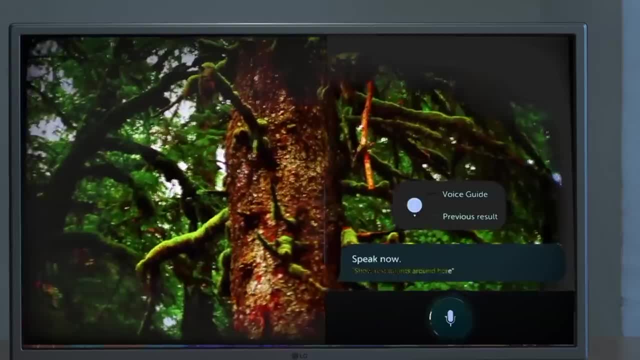 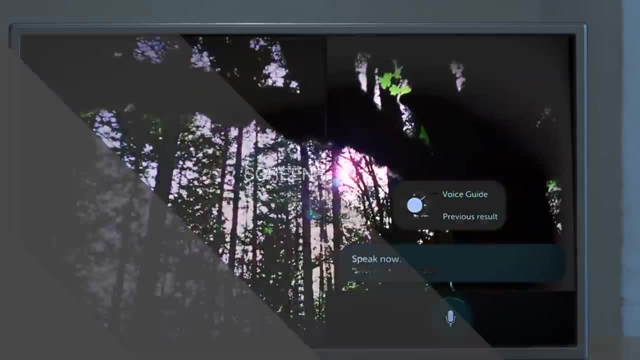 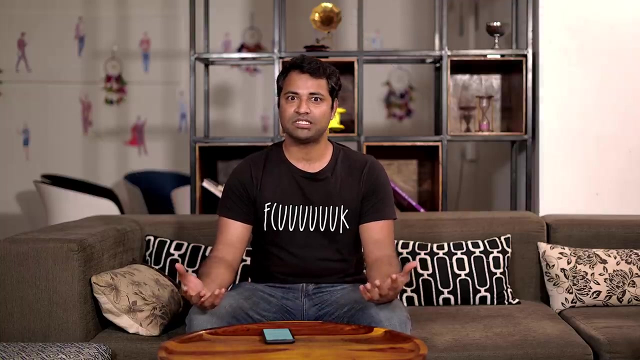 Trust me, it works really good and it's amazing WebOS. It also supports Google Assistant, but you can control your TV only if you have an LG Magic Remote. Another common aspect that you probably see in most smart TVs is that they don't have 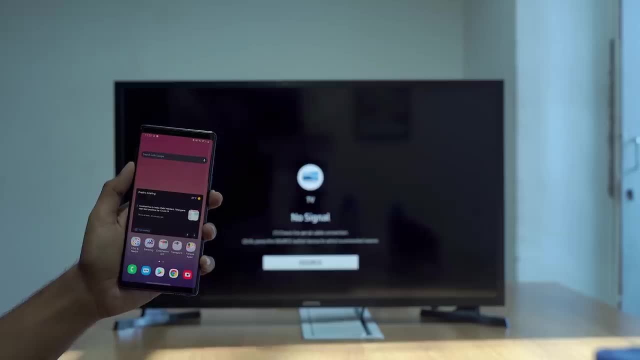 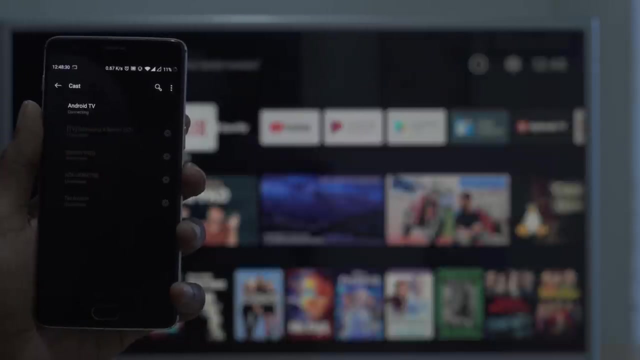 screen sharing. In Tizen OS you can easily cast from your phone to your Samsung TV And if you have a Samsung device, you can cast it with your Smart View feature and you can even cast your content. Android TV uses the Chromecast tech to screen mirror. on your Android smartphone You can. 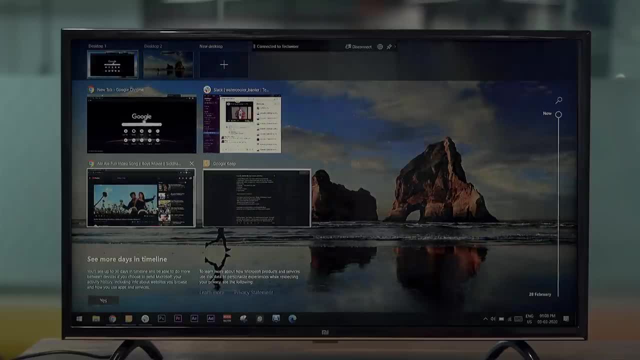 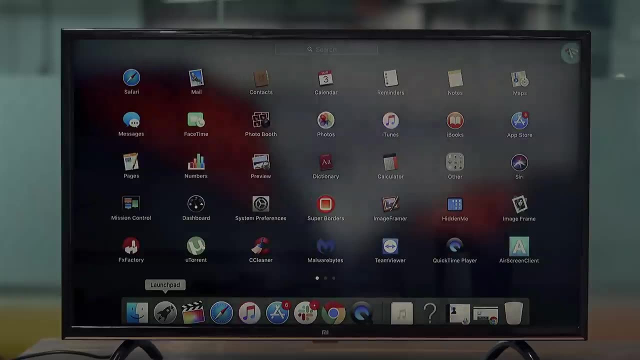 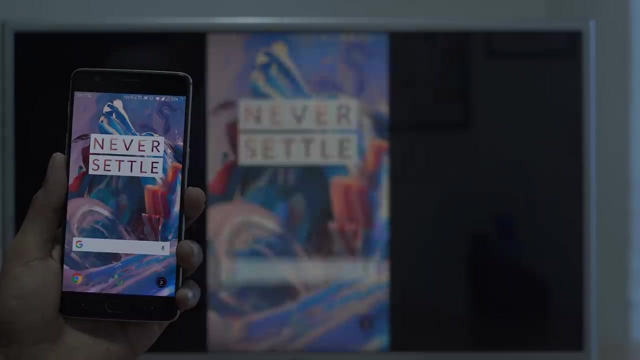 also mirror your computer by using the Chrome browser extension. Also, if you want to mirror your Mac screen, you can use third-party apps like AirScreen to cast Mac screens. WebOS, on the other hand, uses the screen share, which not only casts your Android screen. 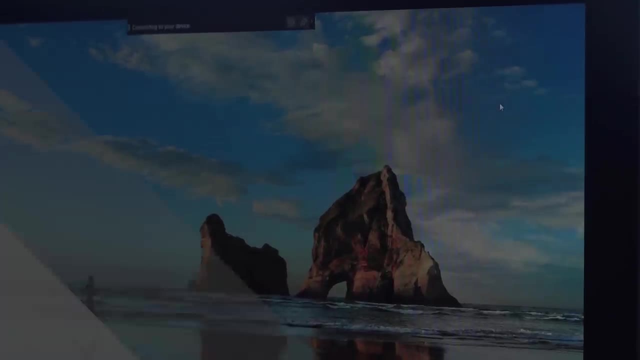 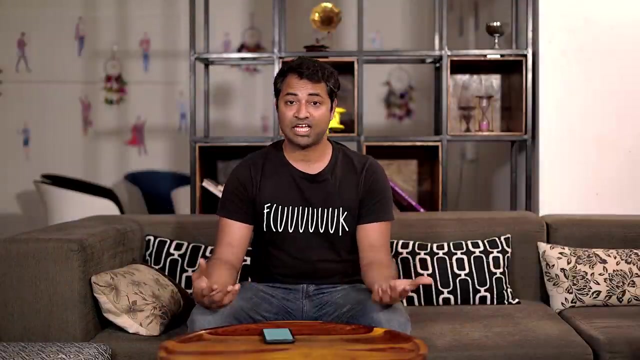 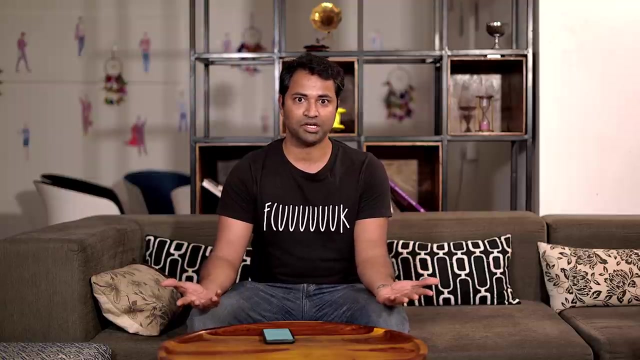 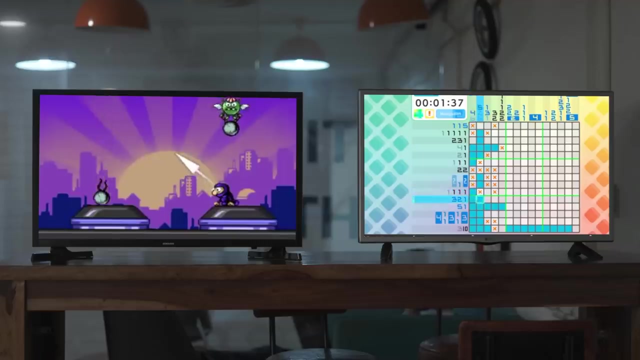 but also any laptop, without having to use a separate app Gaming. Most games that are available on TVs are not exactly console-level games, but they're still pretty good. Some TVs come with actual games. Tizen OS and WebOS both support games, but they have their own store, so you have limited. 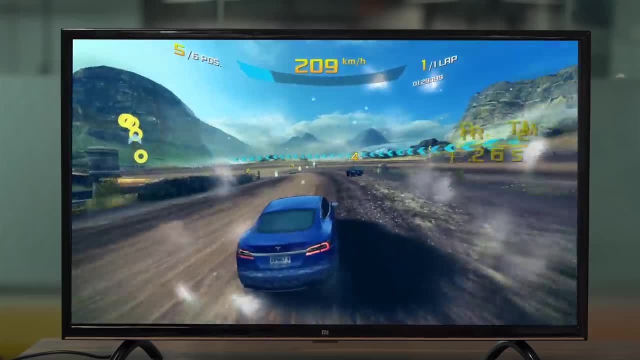 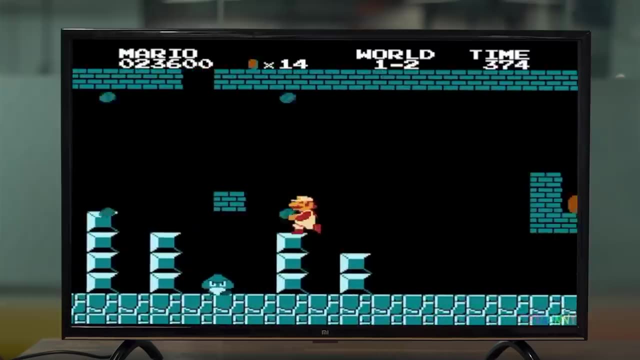 options there, But in Android TV there's bundles of games available, like Asphalt, Badlands and a bunch of others that we've even made videos on. Also, you can sideload any games like Mario and play it with an emulator like RetroArch. 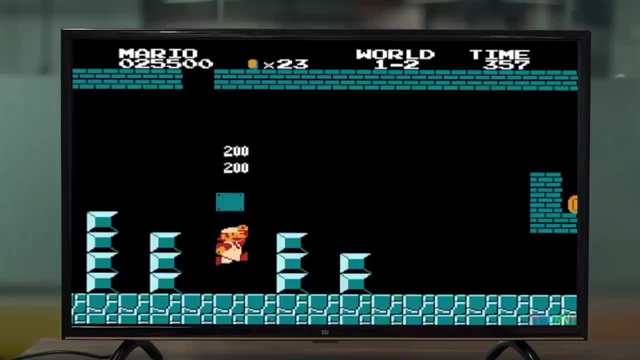 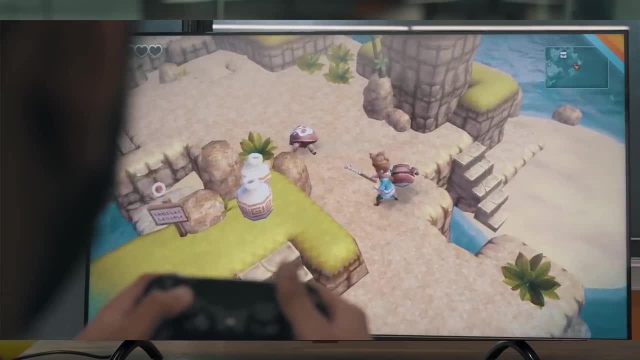 We have a detailed video on that as well, so click on the YouTube cards to watch that. You can also connect to your Bluetooth controller With all systems, but in Tizen OS and WebOS you don't need any extra controller. They only have their basic arcade games. 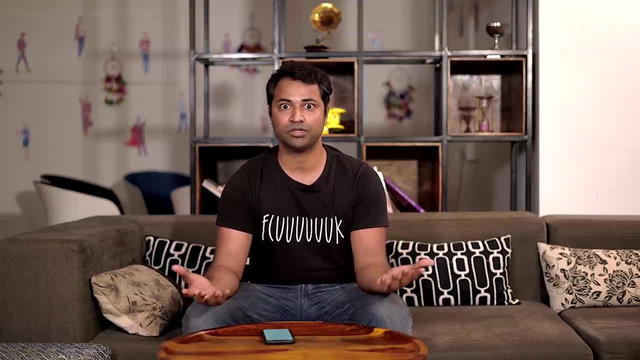 So, finally, which one's the best operating system among the smart TVs that we saw? Well, firstly, pick a TV based on the hardware, like display, audio system and screen size, of course, And after that, if you're looking for a TV based on the operating system that you like, 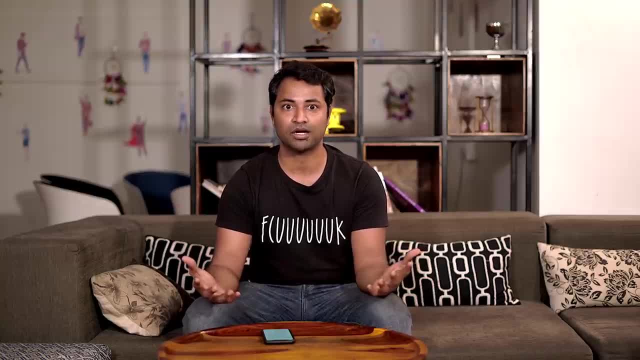 I'd say: go with Android TV OS because it gives you the most bang for your buck, Like apps you know, games and, of course, you can connect it with other IoT devices like Google Home. That being said, if you're already invested in the Samsung ecosystem, just go with the.